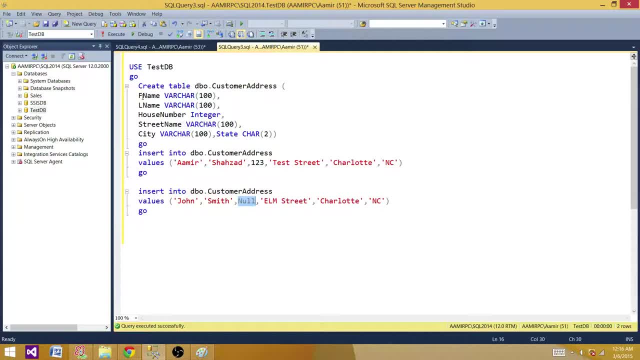 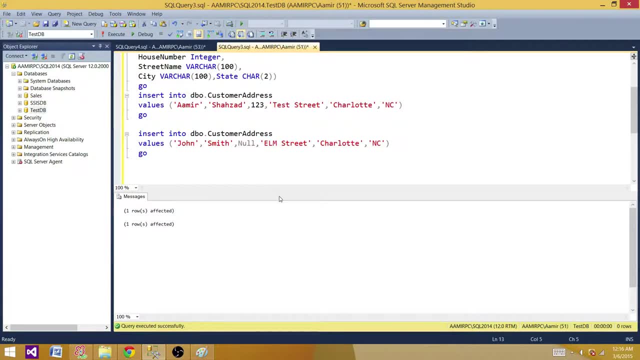 So we have null values there. So let's create this table and insert this value: Execute. So the table is created and Now we can query this table. So let's start from DBO customer address. That's our table. Now what do you see? 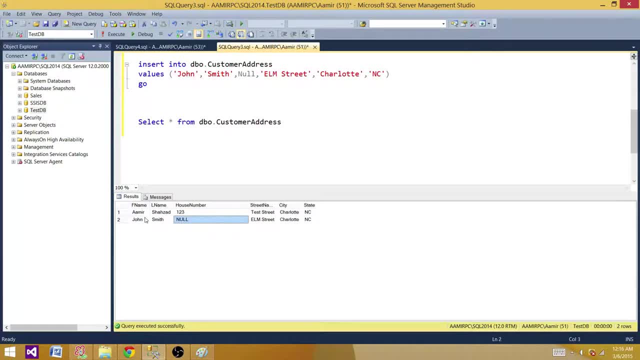 We have a null value in the house number for John Smith. So what we want to do from here? we want to create a complete address by using house number, street name, city and state. So how we can do that. So let's consider. 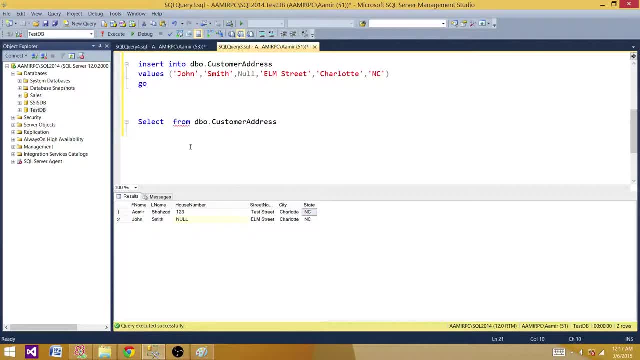 concatenating all of these columns. So we want to do house number and then we want to concatenate with other columns, But before we concatenate I want to put a small space between them. So I want to consider putting space between them. Then I wanna have a street name. 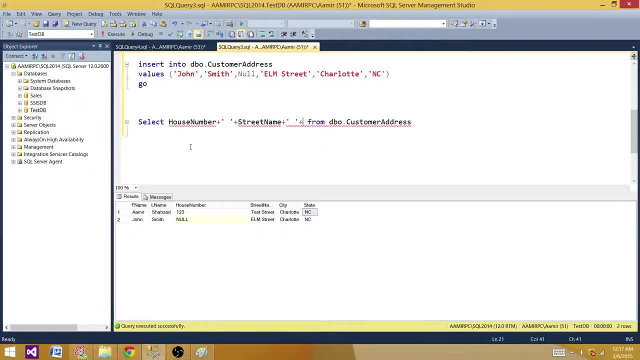 Then again I want to have space between Those columns, city to it, and then i want to have space again and then what i want state: so this statement, my or this sql statement might fail. why? because the house number, in this case what we know. we know that already it is a integer. 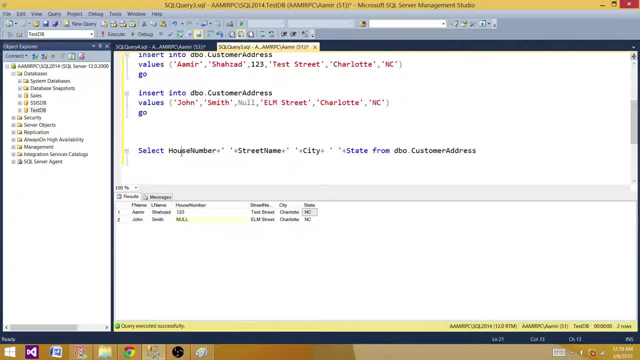 so if this will be string, this will not fail. but in this case it is going to fail as it is a integer, so let's run this one. so what we see here: conversion failed when converting the worker value test street to the data type integer. it is not able to convert. so what we have to do here? 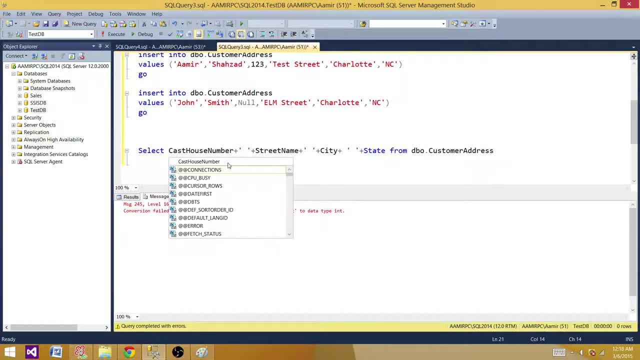 we have to convert so we can cast or use the convert function as worker or char, whatever we want here. so let's consider this one to be varchar 10. so so now our house number is converted to this string and we can use the plus sign to concatenate all the string values, or 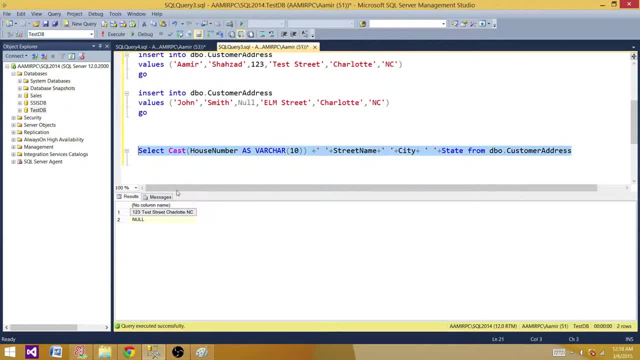 string columns. so here run the query and what we see here, and i can give the comp as name, as full street address. so now we have. so what we see here. let me put the s asterisk here, so i'm getting all the column, then i'm creating. 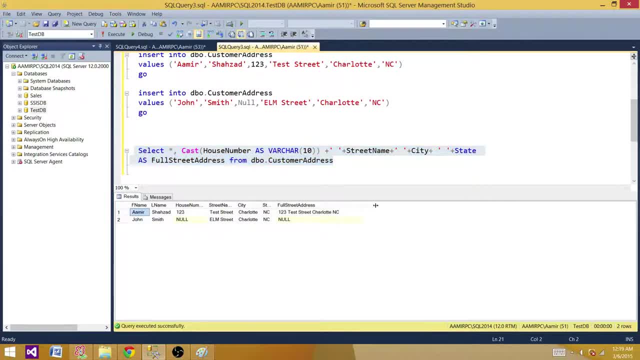 the next column. so what we see here: because of this null value, when we concatenate these columns or the values of these columns, what happened? it converted to the null. when we are using the default settings of the sql server, we are not implementing any or changing the setting on server level or database level to 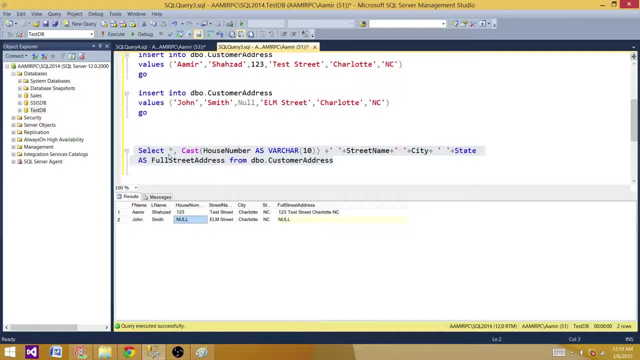 handle this situation. so with the default settings of SQL server, if there is a null value in any column and we will add that or concatenate that by using the add sign, what's going to happen? it is going to give us a null value. how we will address these situations if we use a plus sign, so in: 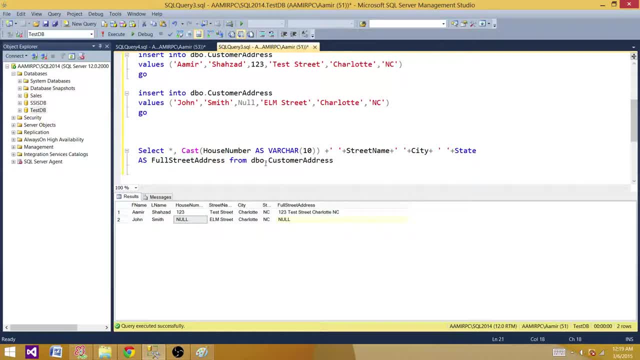 those cases what we use, we use is null, so we say is null. we try to find if there is any null value and we want to replace that. so we can replace that one with the space here or blank, so that way we can handle these situations. now you 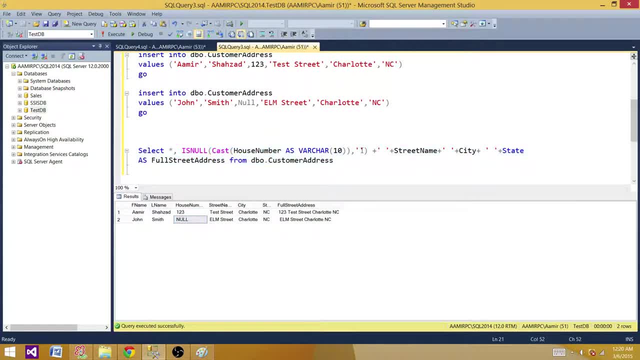 see here this null is converted to the space and that's how we got this result. but see here we are doing a couple of things. we have to have a user is null for all of the other columns that we are going to use, so we have to have a user. 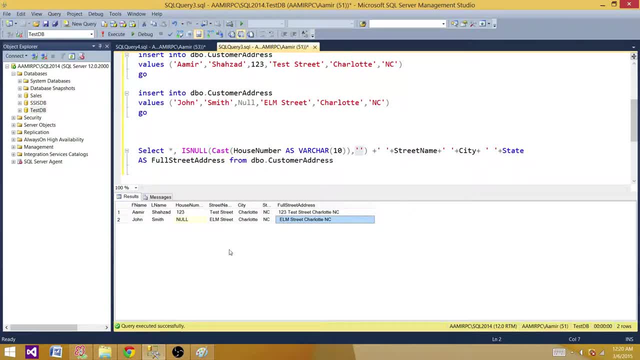 for all of the other columns that we are going to use, so we have to have a user as well. there could be a possibility. we have more records here and there would be. any of the column can be null, that can convert or that can give us the. 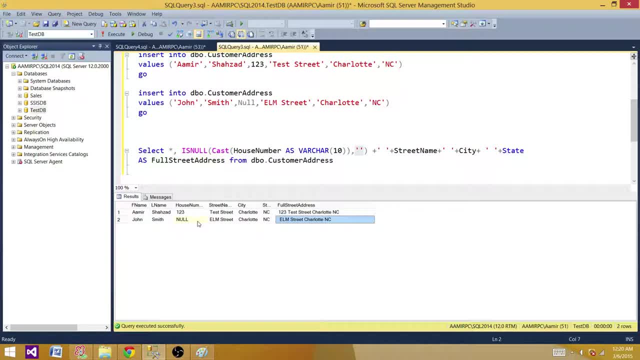 wrong information. it will be only given us a null values in the full street address with the concatenate. let's take the same query and convert to concatenate function. now, in this query we will be using concatenate, so one thing we will be using here. let's remove this part. 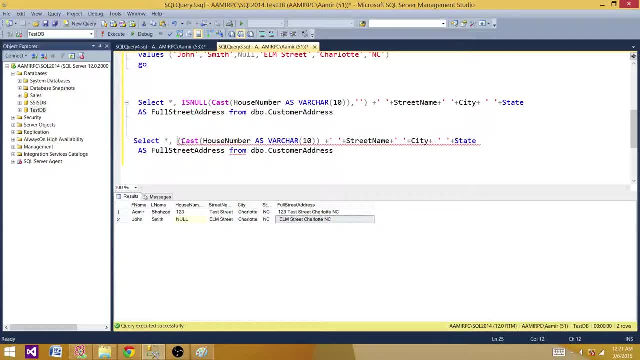 still, we have to cast or convert the house number to the watch, our stringer and I'm you going to use the concat function here, and then we have to put another parenthesis around here, and here the concat function work like this. so you have to have right concat and 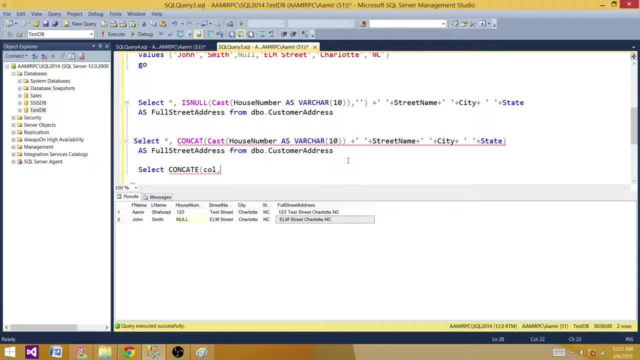 then you have to provide a column, one of value one or whatever. then you provide value two and you keep providing all those values. so that's how we are going to build our full address here. so we'll use in same concat function here. then instead of the plus sign we will be using the comma. here again we will be. 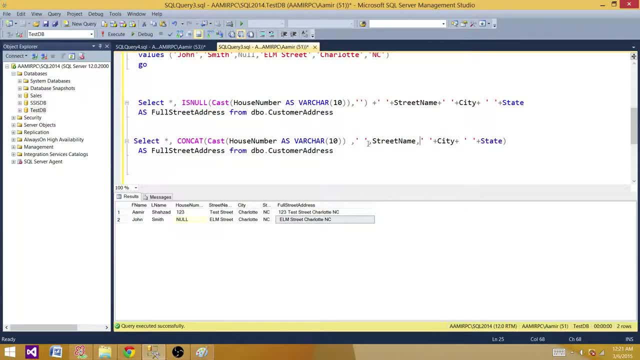 using comma, and you see that I'm still adding the blank space between those columns, so that's also allowed to use the as a hard code values. but for the concat functions wherever you want to write something up if you want to write at the end, sometimes a is a complete address, or 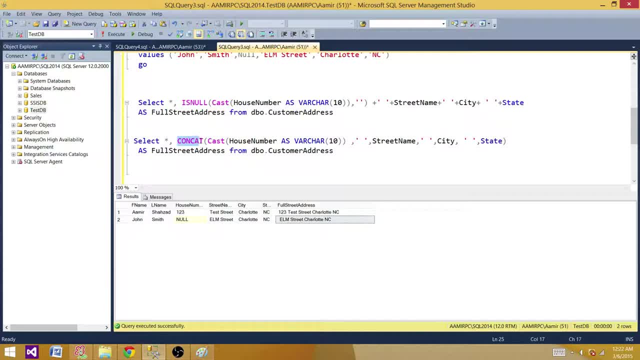 whatever. so you can write it. so can cat function? then you are casting the house number as a worker because can care to accept the strings, and then you have to put the comma and then another value, and then you have to another other values. so keep adding those values or whatever is required. 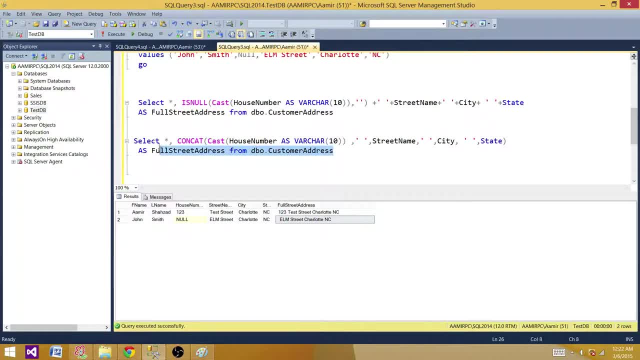 to concatenate. so this is how you are going to build your string. so select here. so what is happening here? so even we have none here and we did not use is null function to replace the value null value with the empty string or something still. we are. we are getting a address without a null, so concat function will. 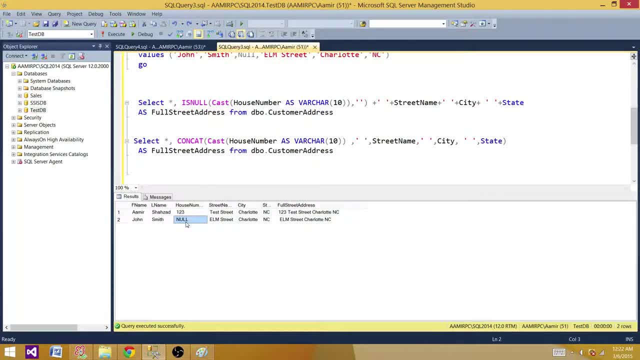 not consider null. it will eliminate the null values but concatenate a all those other values and they give us the output. so that's the difference when you use the plus sign and concat. so in the plus sign, if you are using plus sign to concatenate, you have to make sure you are converting the null values of the. 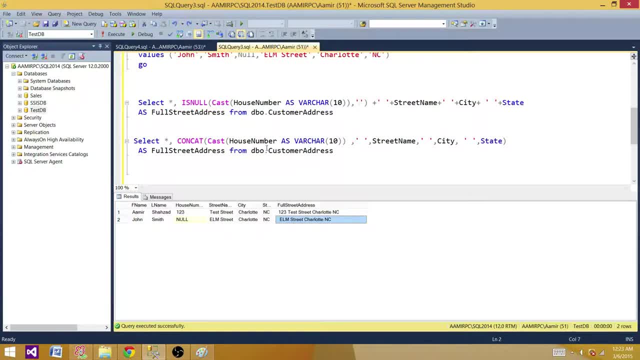 columns to some blank space or whatever you want, and then in the concat you don't have to worry, that will be eliminated. so thanks very much for watching this video and I will see you next video. you.